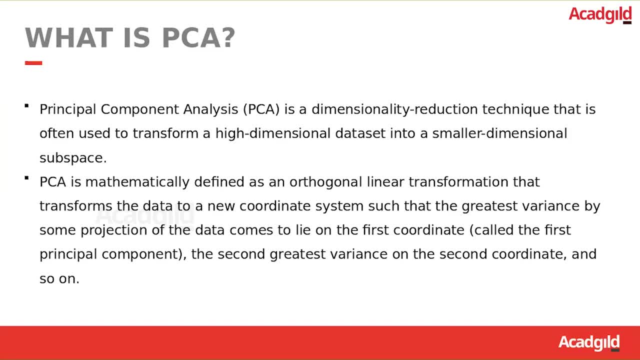 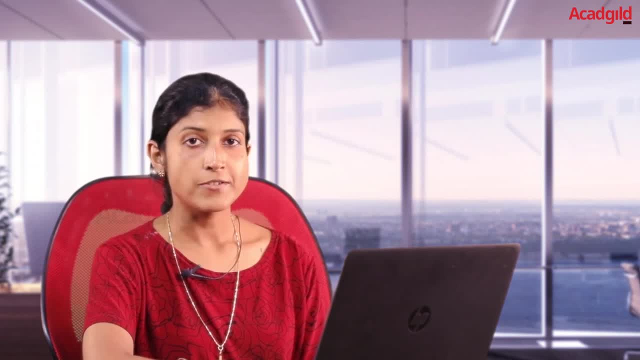 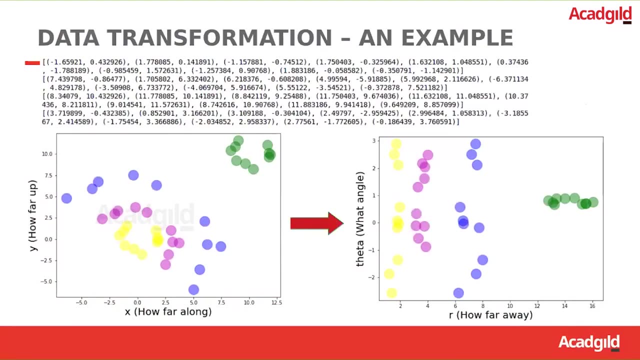 of the data comes to lie on the first coordinate, called the first principle component, the second greatest variance on the second coordinate, and so on. So let's look at What data transformation can do for data and for machine learning algorithms. Let's assume that we have this data set to deal with. 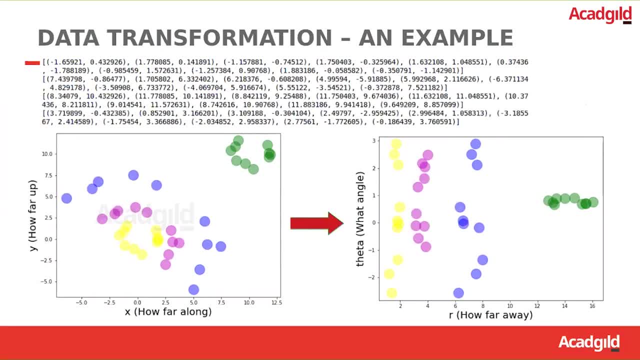 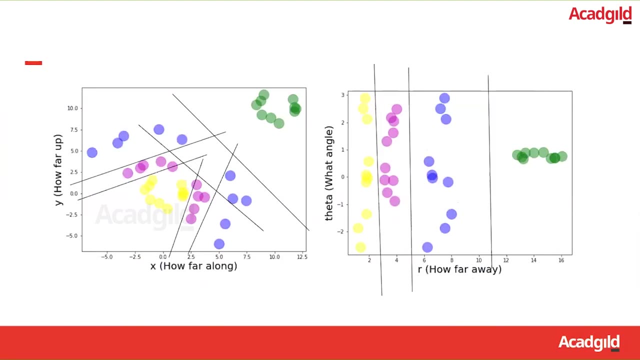 The original data set is on the left. You can see that, in order to classify this data set, it's hard to draw hyperplanes that separate the different classes out. The different colors in this data set correspond to different classes of data, But if we were to draw lines, we would have to draw so many lines that actually separate. 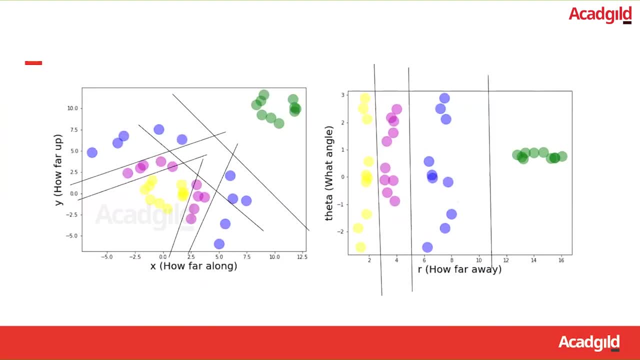 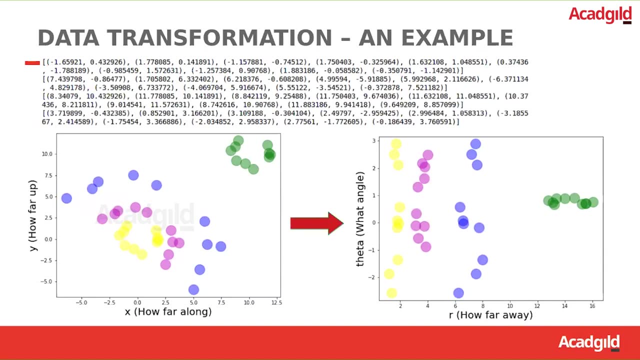 the data from one class, One class and another. The data on the left is expressed in Cartesian coordinate system. Each of these coordinates signifies something. The x coordinate signifies how far along each data point is, And the y coordinate signifies how far up it is. 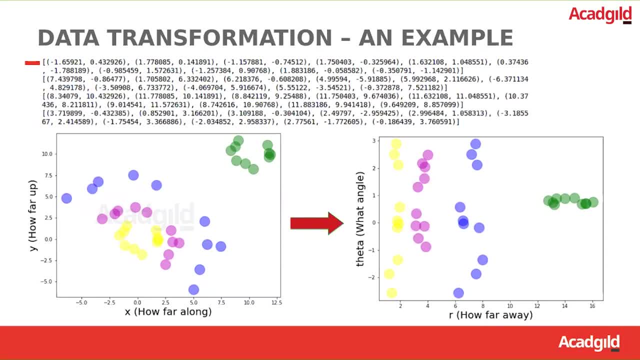 If we were to express the same data in a different coordinate system, which is a polar coordinate system, using r and theta, we see how the data is distributed in a different way. So let's look at Now in order to classify the data. if we did this transformation, it becomes much easier. 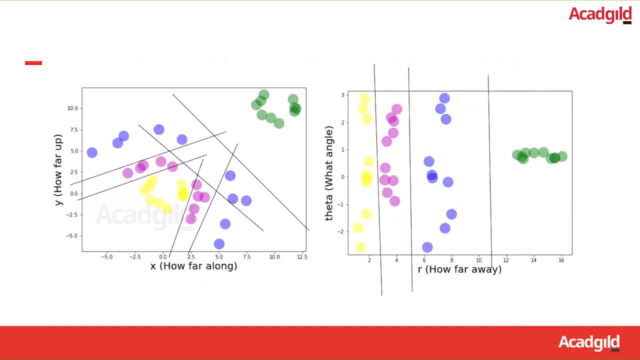 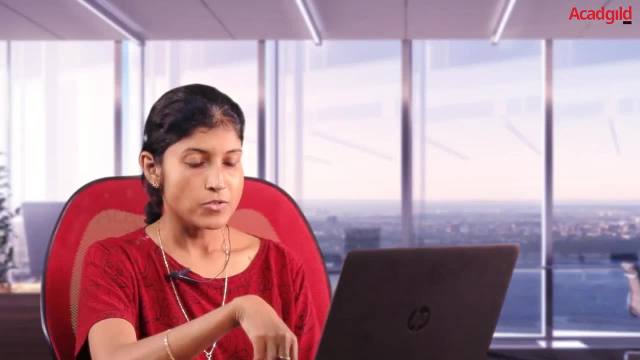 to do that, We just have to draw three hyperplanes and we are able to classify the data into four classes, which was not possible when we used it in the Cartesian coordinate system. So this is what data transformation does as a pre-processing step for machine learning. 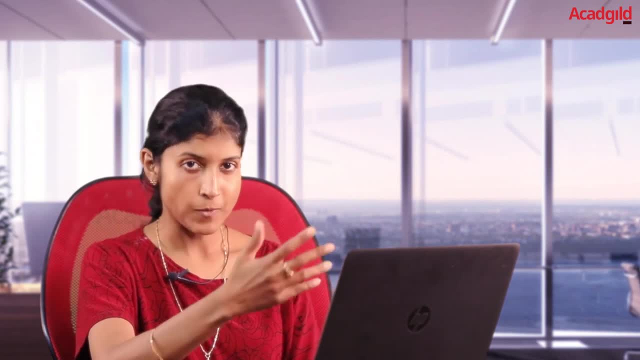 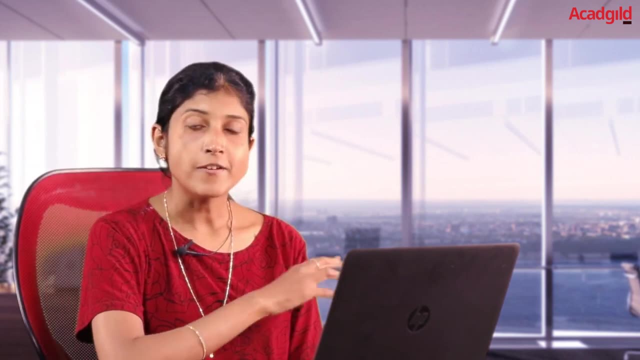 algorithms. It expresses the data in a different way, in such a manner that the task that the machine learning has to accomplish is accomplished easier. Let's look at- Let's look at a rough example in real life in which something like principal conflict. 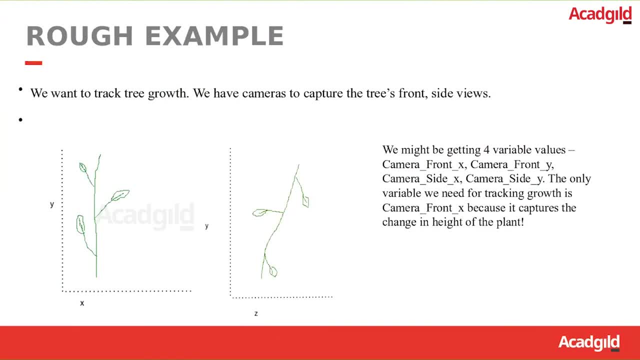 analysis will help. For example, let's assume that we want to track plant growth. We all know that plant growth typically occurs in the vertical direction. So now suppose we had two cameras, one facing the front view of the plant and another facing the top view of the plant. 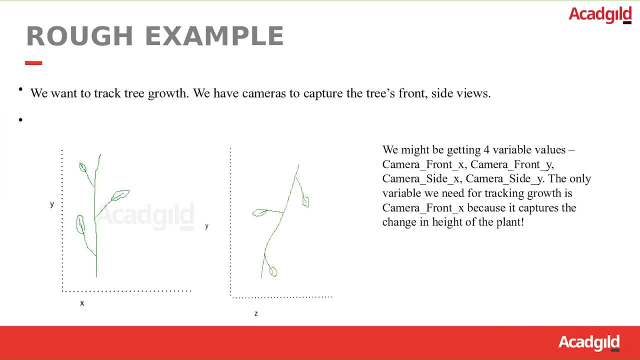 Each of these cameras give two dimensional data about the plant. The front facing camera gives the x and y dimensions and the top facing camera gives the y and z dimensions. Of the four dimensions that we get from the two cameras, the only dimension we actually 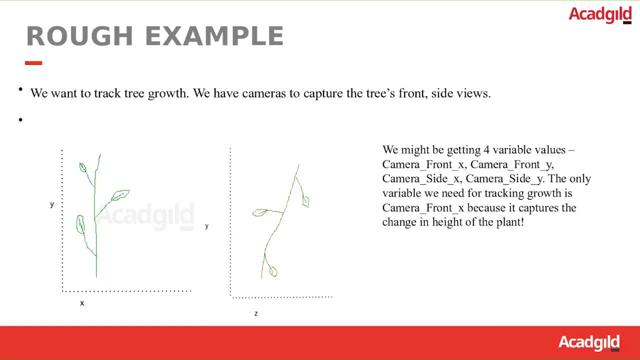 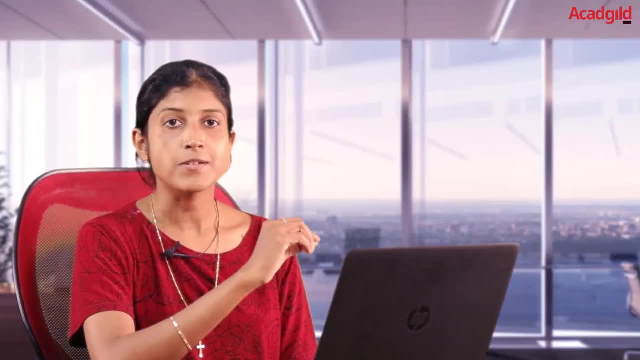 need to get information about plant growth is the y dimension from the front facing camera. So now we see that we have four dimensional data, which can be reduced to just one dimension in order to get information about the phenomena that we are actually interested in. 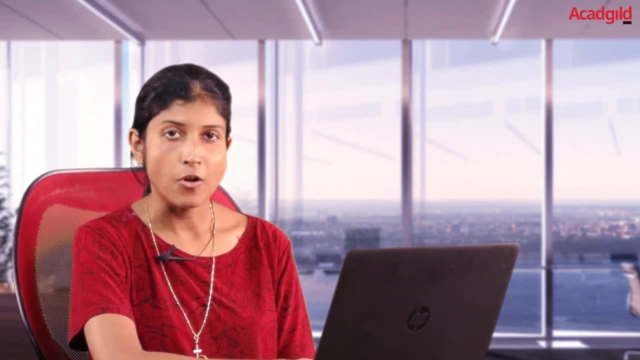 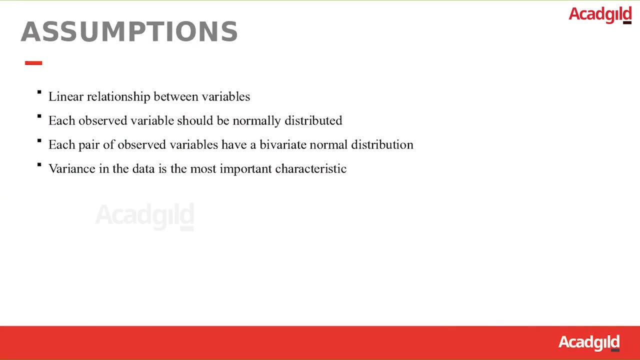 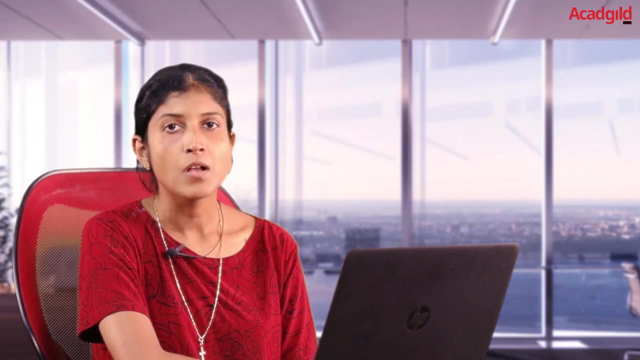 So some assumptions that PCA makes about the data that it is used on are that the variables are all linearly related to each other, That each variable is normally distributed And that variance of a particular dimension is the most important and interesting characteristic of the data. 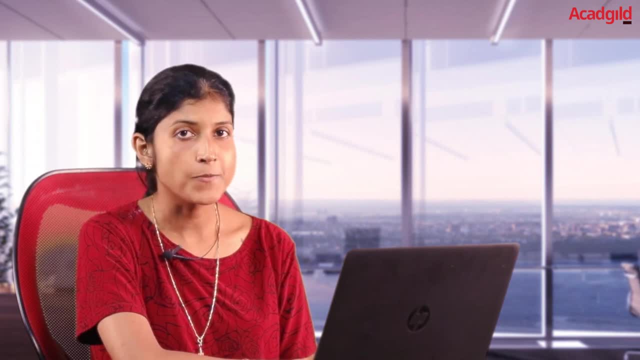 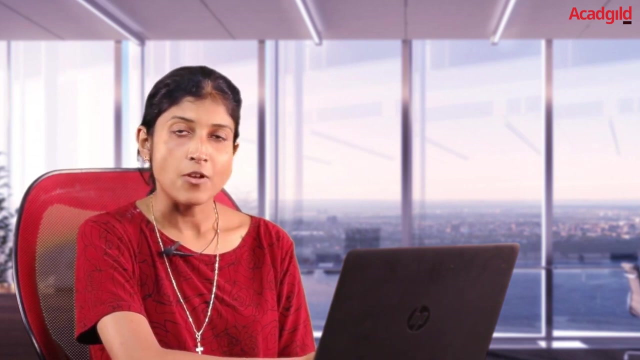 So we've already seen that principal component analysis is actually a data transformation technique in such a way that the data that is in some coordinate system is now going to be represented in a different coordinate system, in such a way that information that is needed for a machine learning algorithm or for any other process is not lost. 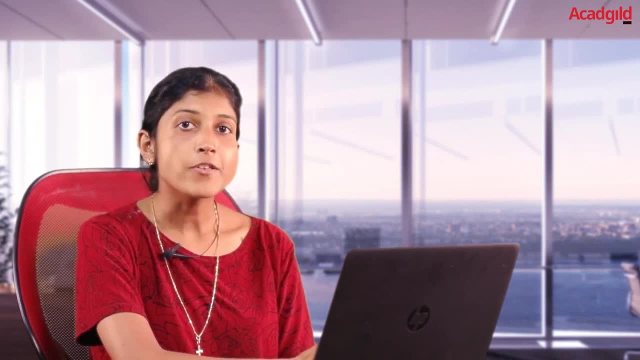 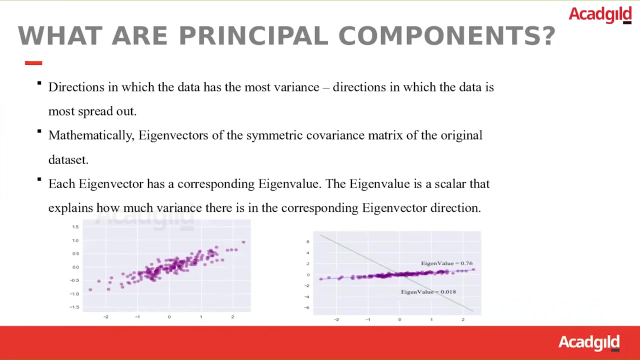 So principal component analysis finds the principal components or the new components, the new coordinates that can be used more effectively to represent the data to the machine learning algorithm. So what are principal components? Principal components are simply the directions in which the data has the most variance, or 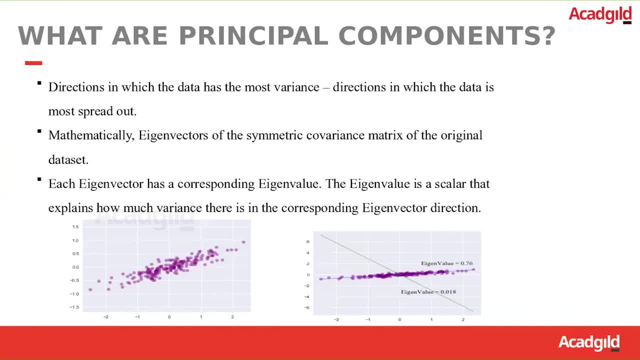 the directions in which the data is the most spread out. Mathematically, it is the eigenvalues and eigenvectors of the covariance matrix of the data set, Each eigenvector which corresponds to the direction in which the variance is greatest in the data set. 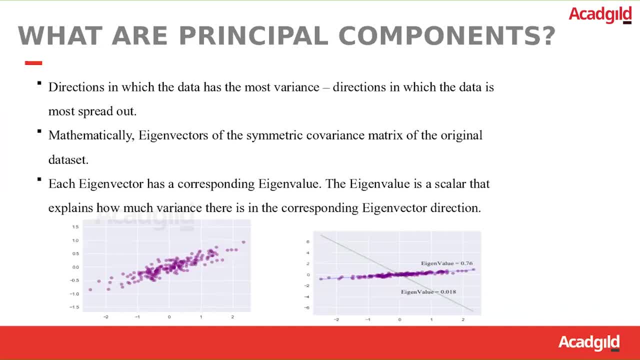 Has a corresponding eigenvalue, which signifies the magnitude of the variance that each dimension expresses. Now let's look at the data that has been plotted on the left side of this figure. We see that this data, the two dimensions, are linearly related to each other and that 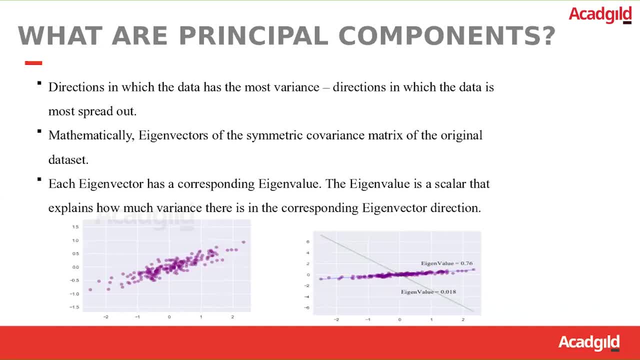 they are somewhat spread out. So now we want to find out the directions in which this data is actually most spread out. So you can see that, after plotting the eigenvectors, they lie around the directions of the most spread, the greatest spread. 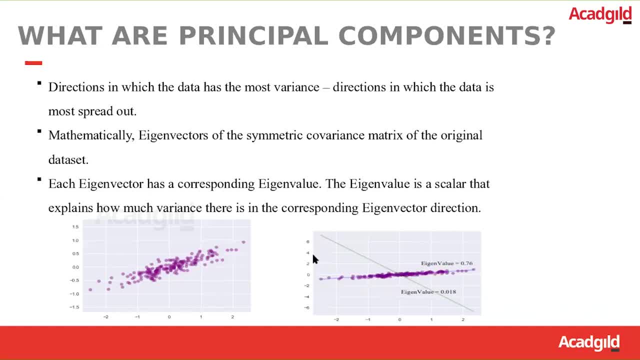 And you can see that the eigenvalues that correspond to these two lines that signify the eigenvectors, gives us some idea about how much of the variance each of the dimension represents. So the eigenvalue here is 0.76 signifies that this direction contains 0.76 of the variance. 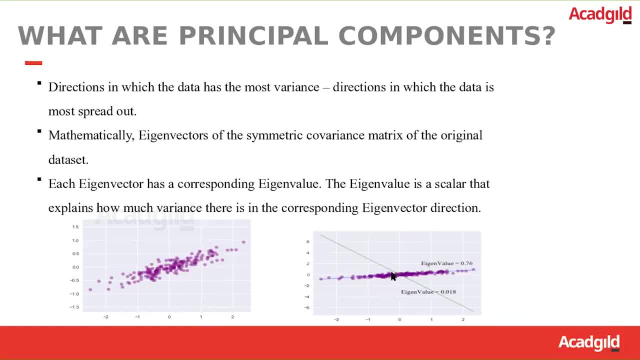 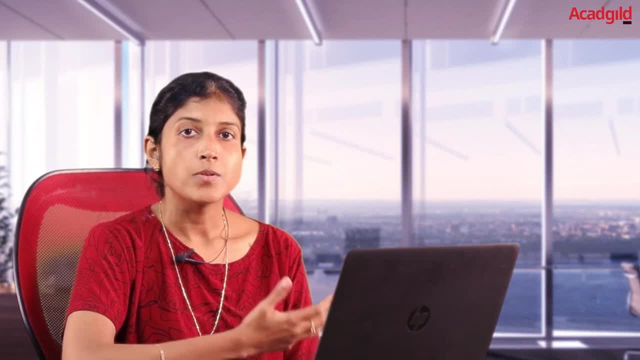 of the entire data set, or 76%, and this direction only contains 1.8% of the total variance in the data set. If we wanted to do mathematically, If we wanted to compute the variance, If we wanted to compute the variance, 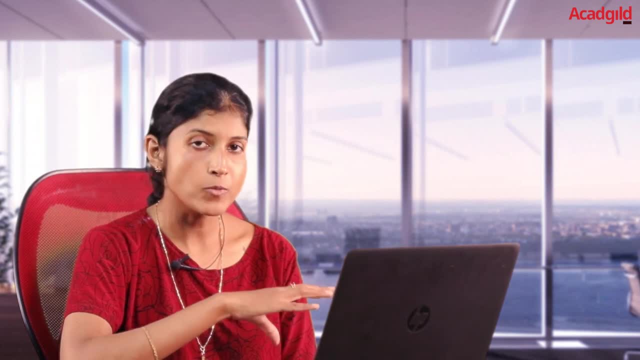 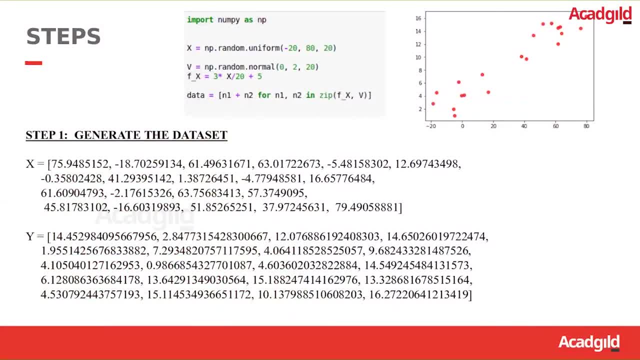 Let's just first generate a data set. So the data set that I'm going to be using is given here, And I plotted it also to show that there is a linear relationship between the variables X and Y that describe the data. I've given you the code, also here in Python, which was used to generate this data set. 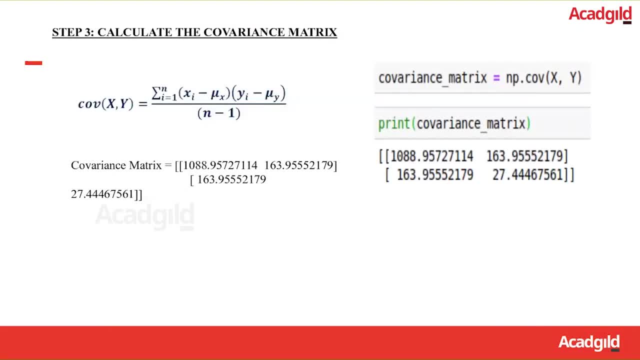 The next step would be to calculate the covariance matrix. The covariance generally is calculated as the sum of all Clap-альные. So here in Python we have the Covariance matrix. So I've done that- of the products, of the difference of each variable from its mean divided by 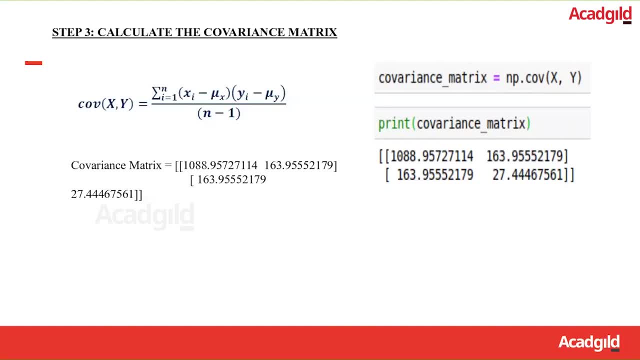 the number of samples that were used. So it's a symmetric matrix in which on both sides of the diagonal we will have the same elements. So the Python code to calculate covariance matrix is simply to use the cove method, which is found in the numpy package. So once we calculate the covariance matrix and print them out, 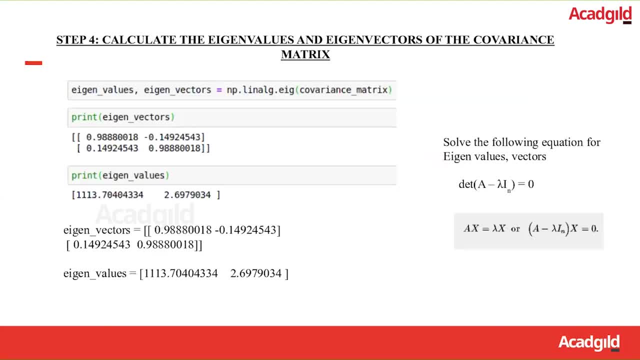 we get these values as shown in the slide. The next step would be to calculate the eigenvalues and eigenvectors of the covariance matrix. So how do we calculate the eigenvalues? For calculating eigenvalues we use the equation given here: Determinant of A minus lambda I equals 0 where A is the. 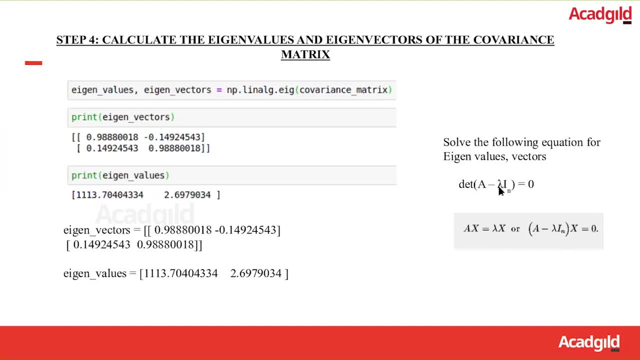 original data set. lambda would be the eigenvalues that we are trying to solve for, and I n is the identity matrix. The n here signifies the order of the matrix. Once we solve for this, we get the eigenvalues and using the eigenvalues we get the co-variance matrix. So the co-variance matrix is 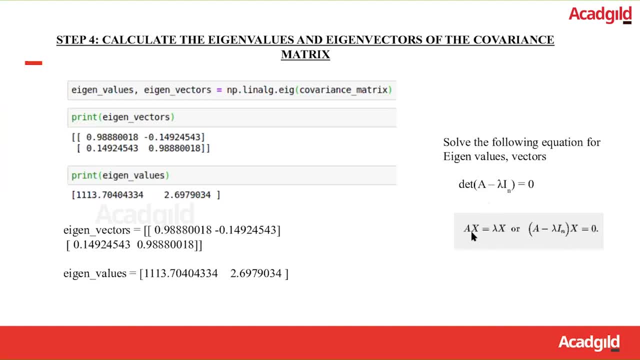 the eigenvalues. we can get the eigenvectors by using this equation: A: x equals lambda x, where A is the data set, lambda is the eigenvalues and x is the eigenvector that we want to solve for. We can calculate the eigenvalues and: 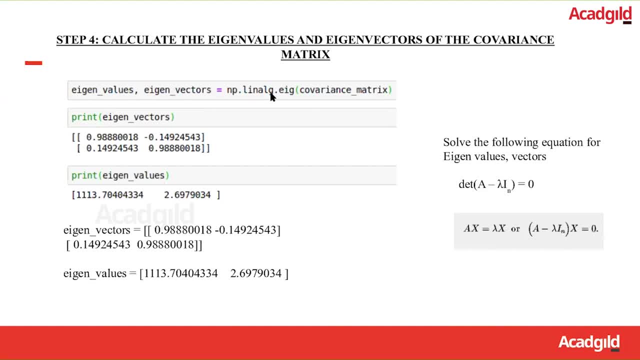 eigenvectors using numpy's linear algorithm, dot eigenmethod, and we call this on the covariance matrix. We can see here that we have two eigenvectors and two eigenvalues. This is because the dimensionality of the data set that we were dealing with was 2.. We had x and y as the co-variance matrix and we can see: 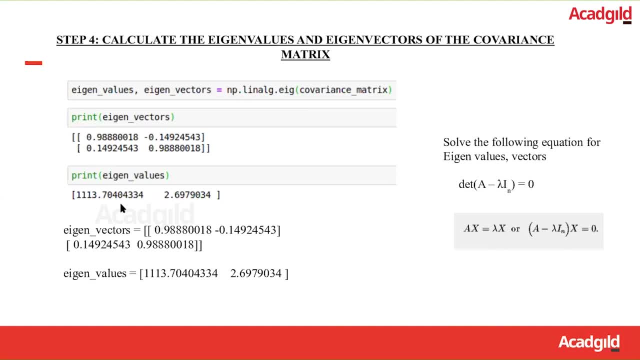 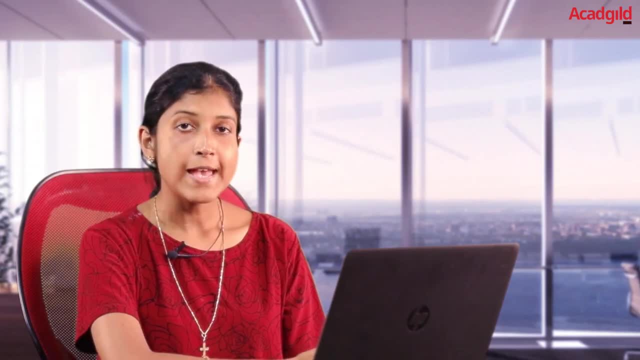 y and those were the dimensions of the data. and here we have two eigenvalues corresponding to the two eigenvectors. that is got from the two dimensional data set. So why do we need PCA? PCA has several applications. One of them is compression. We can see how that is, because data that is originally having 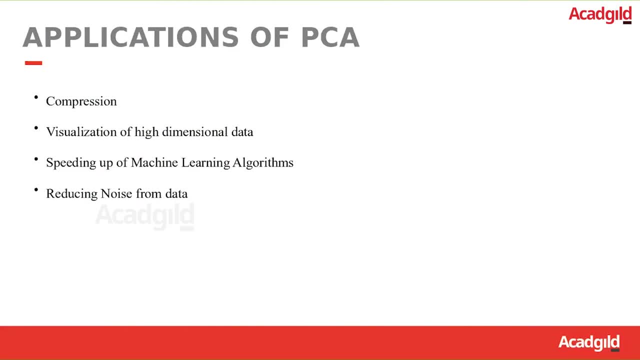 higher dimensions is now represented in a lower dimensional subspace, So obviously the amount of data that is required to transmit the same amount of information has become low now because of PCA. It also has several other applications, like speeding up machine learning algorithms, visualization of higher dimensional data sets and 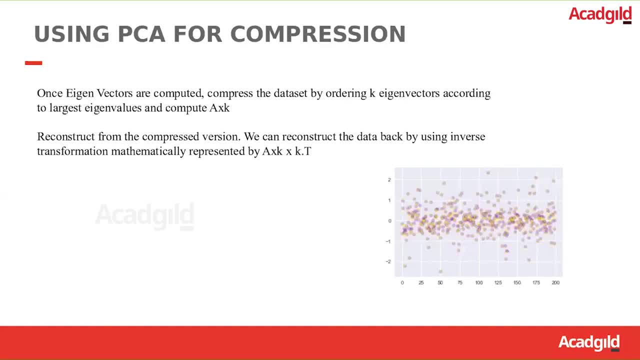 reducing noise. So let's take a brief look at how PCA can be used for compression Once the eigenvectors or the principal components are computed, the data set can be compressed by ordering k eigenvectors according to largest k eigenvalues and the matrix A multiplied by k can be computed. Once that is computed, that will 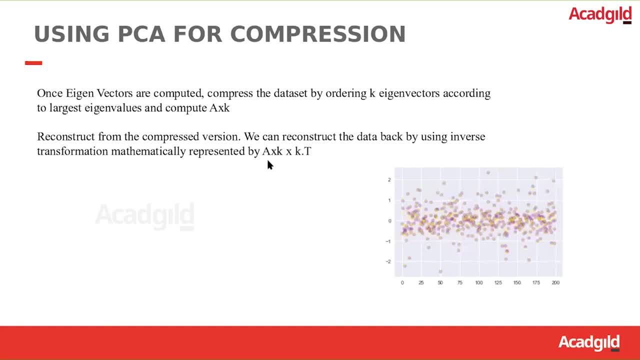 represent the compressed data set set. If we wanted to reconstruct the data from the compressed version, we could do that by multiplying A with K and then multiplying that with K. transpose where all these multiplications are matrix multiplications. We can see from this: 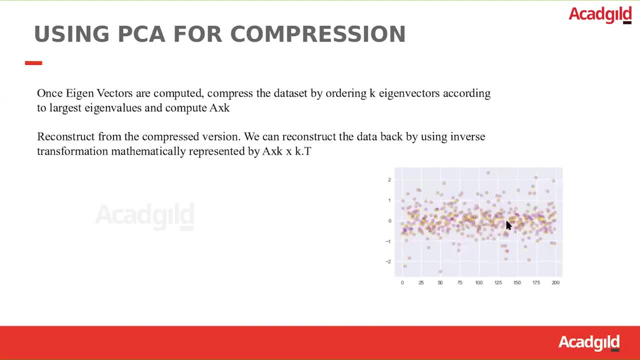 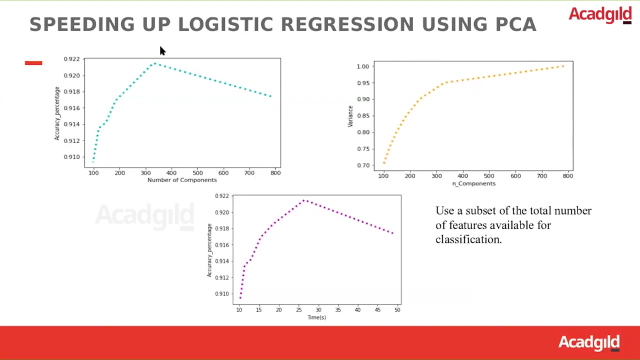 figure here, which is a scatter plot of the original data and the reconstructed data, that the compressed data and the original data. they all look very similar. That's why they overlap so much. So the graphs here show how using a subset of the total number of features available for classification has helped. 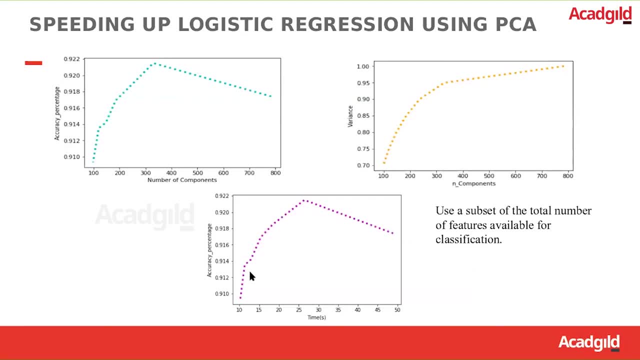 this particular instance of logistic regression to conserve on the amount of time that's required by using fewer dimensions. So the total number of dimensions available was something in the order of 800, but we see here that accuracy does not get worse because of using a fewer number of dimensions. This 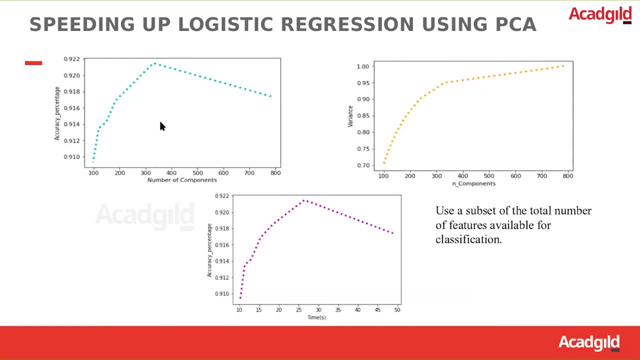 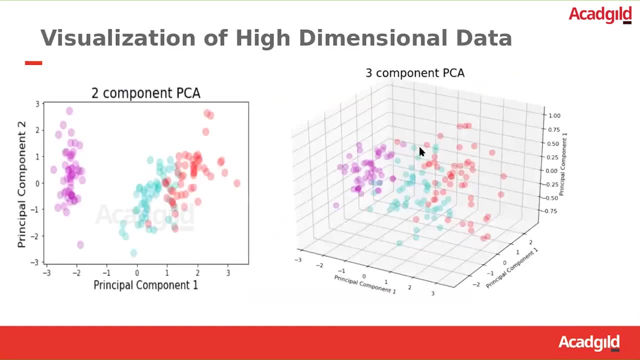 way of selecting the fewer dimensions that was enough to represent the data set was done by using PCA. Another example here is how reducing the number of dimensions can help visualization of data. So this is a three-dimensional data set. this is a two-dimensional data set. 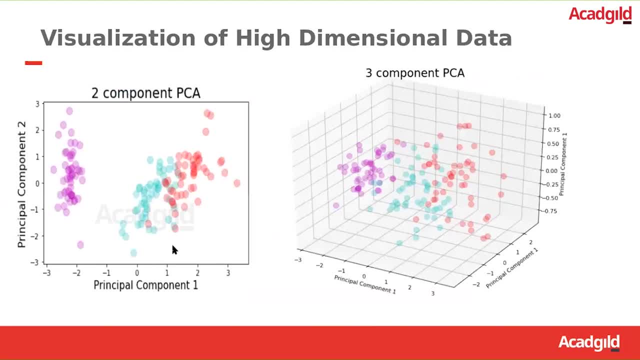 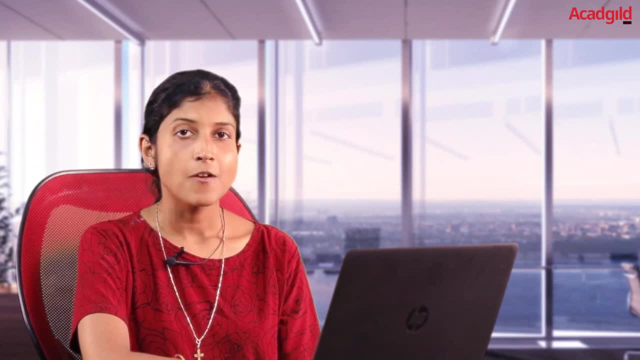 we can see how the classes are separated much more clearly when we have fewer dimensions, and this is also possible with PCA. Thank you for watching this video on principle comfort analysis. For more videos on machine learning algorithms with Python, please subscribe to our Channel. 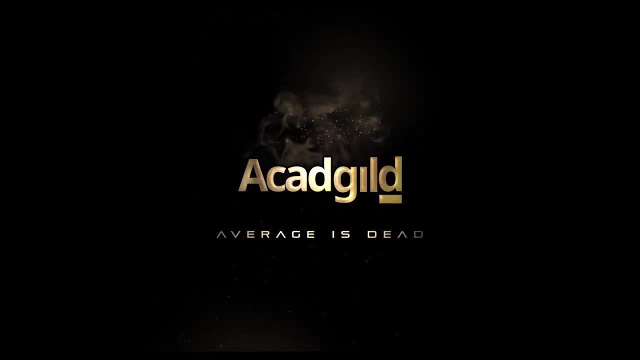 A CAD Count: Average. Average Average is dead. 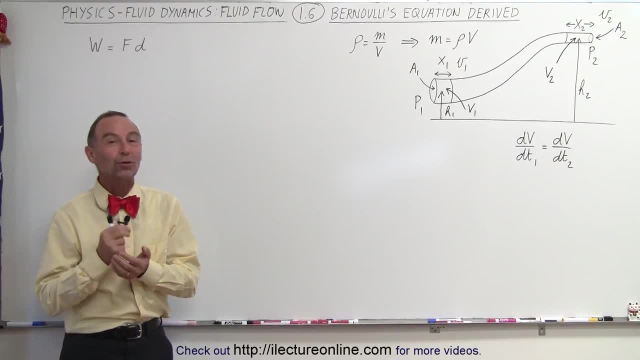 Welcome to iLectra Online. In this video we're going to derive Bernoulli's equation. A number of viewers already have been asking: well, where did it come from? How did Bernoulli come up with this equation? Well, here we intend to show you how he did that. 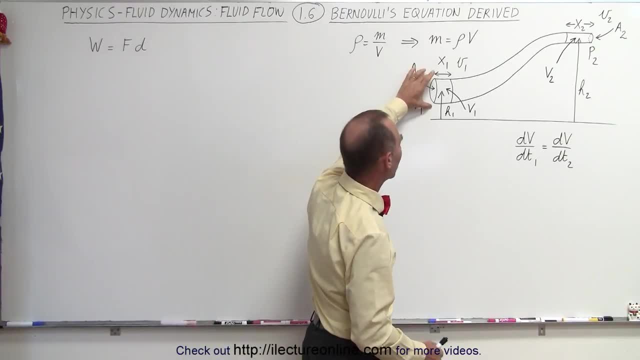 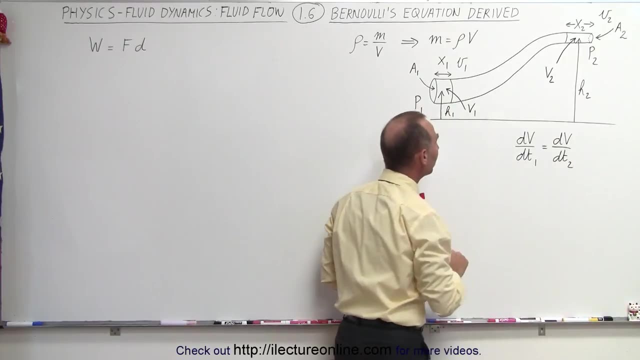 So let's say that we have a pipe that has a larger cross-sectional area here and a smaller cross-sectional area over there. Also, notice that the height has changed as well, but we know that the amount of fluid flowing through the pipe has to be consistent all the way through the pipe. 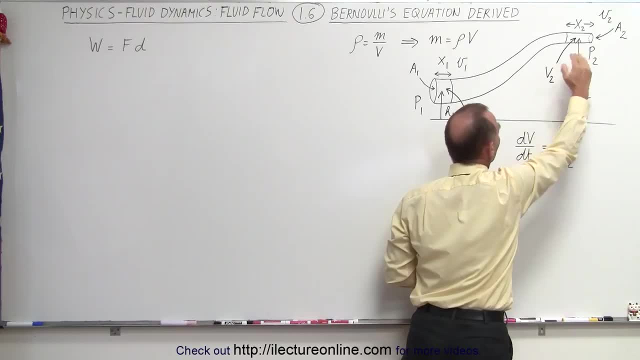 Which means that if the diameter gets smaller, the velocity has to increase in such a way that the amount of volume per unit time that goes to the pipe on one end must be equal to the amount of volume per unit time that comes out the other end. Notice, here we have the cross-sectional area. 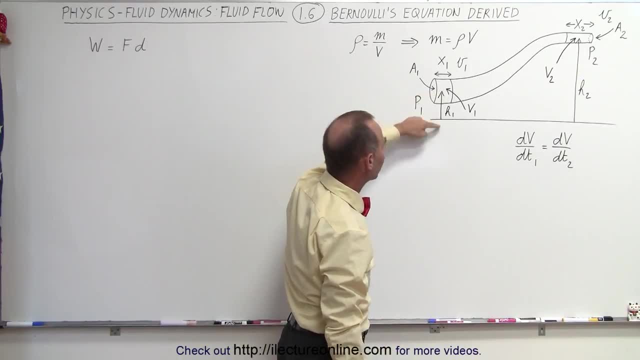 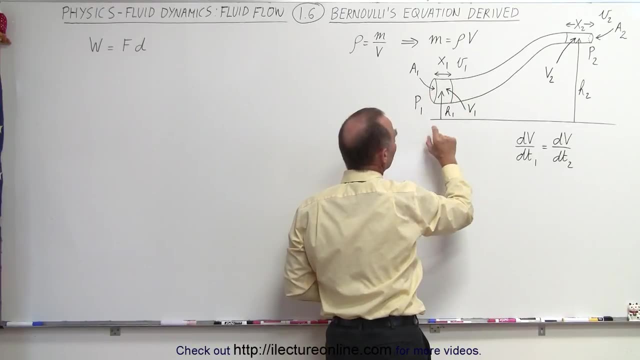 at one we have the pressure. at one the height relative to some standard position h. This is the volume of that particular pipe, That is, the amount of fluid that goes through the pipe, particular element of the pipe. notice: the volume will be equal to the cross-sectional. 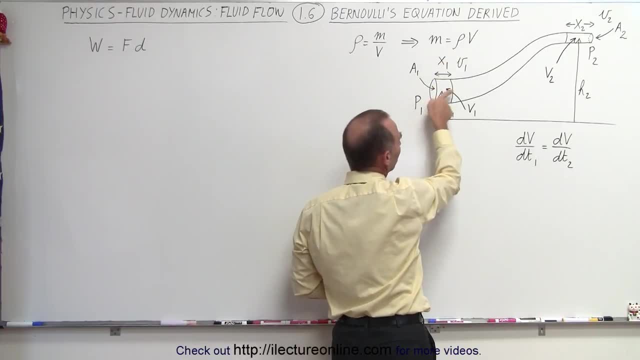 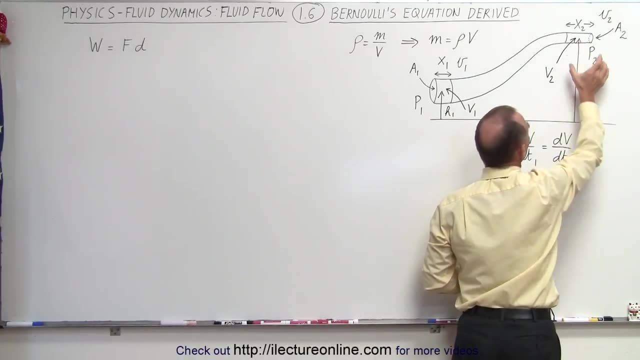 area times the distance x1.. We know that the fluid will flow through this part of the pipe at velocity v1.. On the other hand, we have the height h2.. We have volume 2, but volume 1 must equal volume 2.. Since it has a smaller cross-sectional area, there will be a bigger. 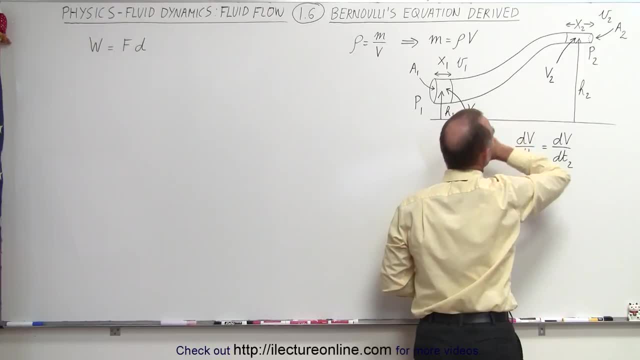 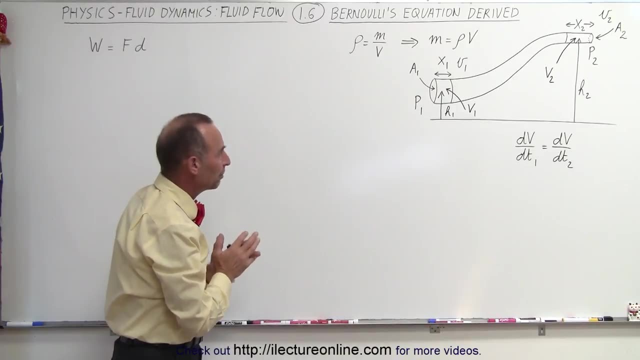 x2.. Velocity 2: there will be larger than velocity 1, and pressure 2 will be over here, Pressure 1 on that side. So now, how do we come up with Bernoulli's equation? Well, we need to have three different.